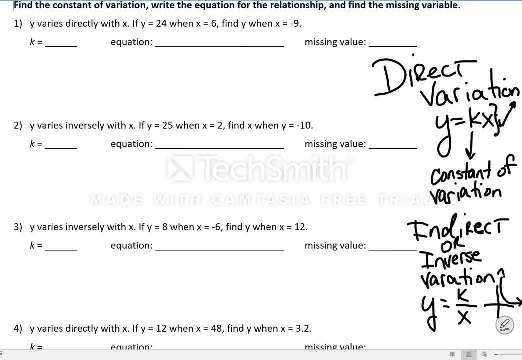 We'll use that here in the next video, or so Now, what I want to do for questions one, two, three and four is I want to use these equations- y equals k over x and then y equals kx, to identify the k which is the constant right. 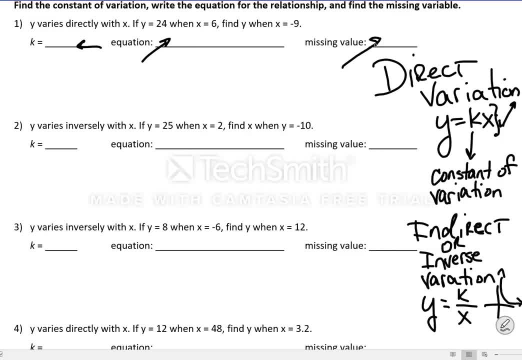 I want to write the equation and then I want to find the missing value. So if y varies directly with x, so my equation is going to start off like this: y equals kx. What I'm going to do is I'm going to take the numbers. 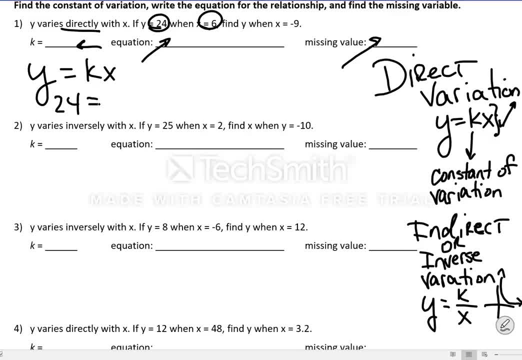 If y is equal to 24 and x is equal to 6, and I'm going to solve for k, which is dividing. dividing k is equal to 4.. So k equals 4.. So k equals 4.. So k equals 4.. 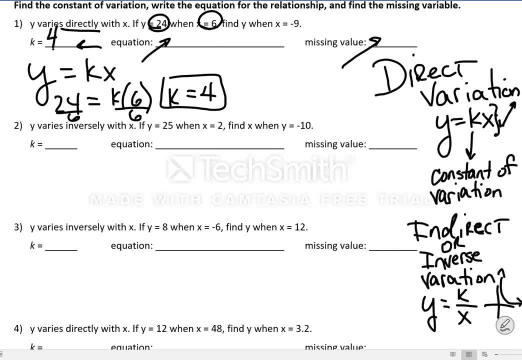 That was easy. Now your equation. this is where it gets a little tricky because we're going to want to do different things. Your equation is the direct or inverse variation equation that is only substituted in for the variable k. So our equation, we said, was y equals kx. 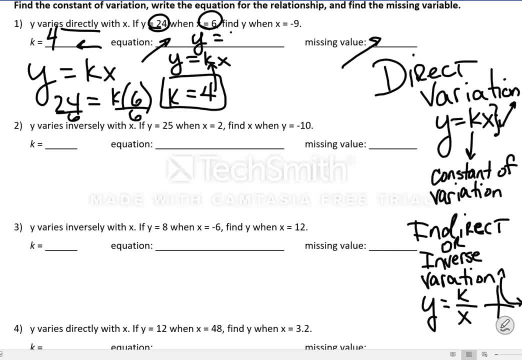 The 4 is k. So when I rewrite this, this is actually: y equals 4x. So my slope, or my constant of variation, is 4.. Now I'm going to find the missing value. So, using the equation that I just wrote, I'm going to plug in, substitute in the negative 9 into x to find out the missing value of y. 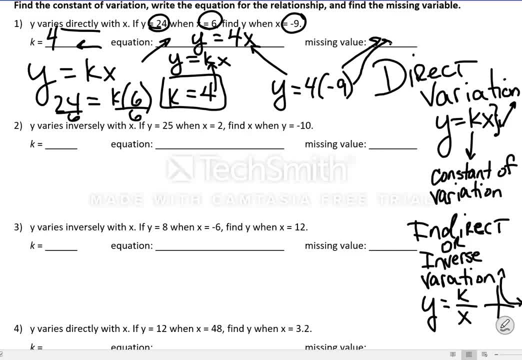 So it's 4 times negative 9,, which gives me negative 36.. And that is how you do a direct variation equation And the k value and the missing value. That's how you do all that stuff. So now I have an inverse leave. 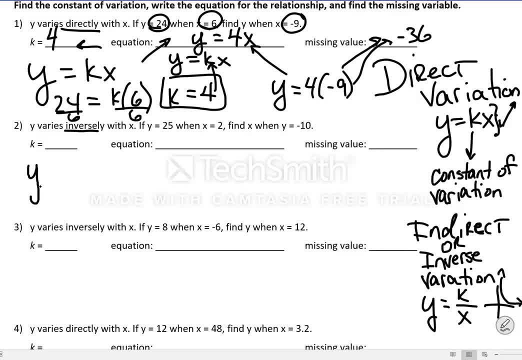 Question: equation. So start with the equation: y equals k over x. I'm going to plug in what I'm given to find my constant. So it's 25 equals k over 2.. And remember this is division. So what's the opposite of it? 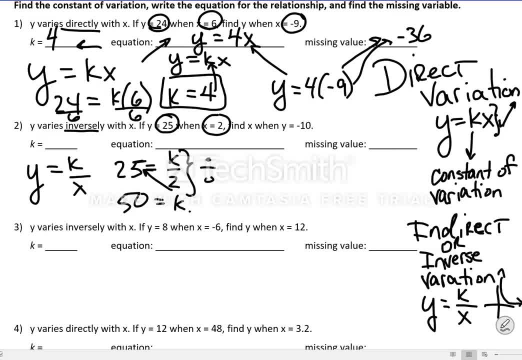 Multiplication. So 50 is equal to k, So k is 50.. So now again, my equation is: y equals k over x, because that's our generic one, And the only thing that I'm changing is the k value. I'm plugging the 50 in for it. 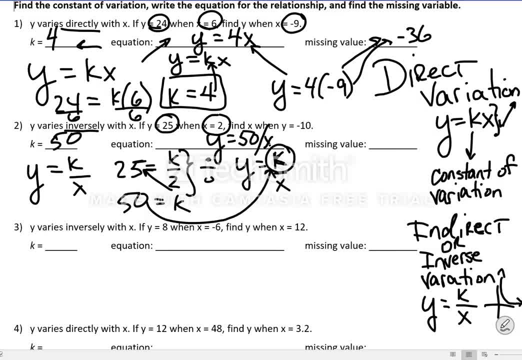 So y equals 50 over x. And then the missing value. I'm going to use the equation I just wrote. So y equals 50 over x. What do I have? Well, I have the negative 10.. So negative, Negative 10 is in, for y is equal to 50 over x. 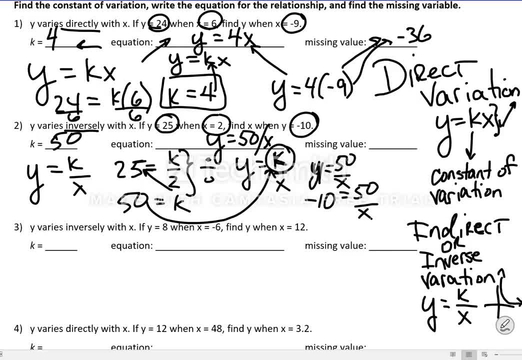 And remember this is a proportion. So I can use the Hart method, cross multiplication, multiply diagonally and then solve your equation. Or what I can do is, if we remember it's a proportion, diagonals, I can switch the values. 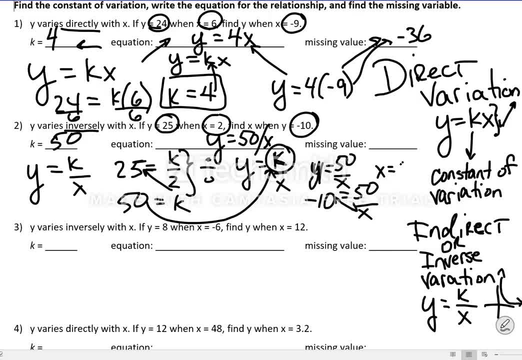 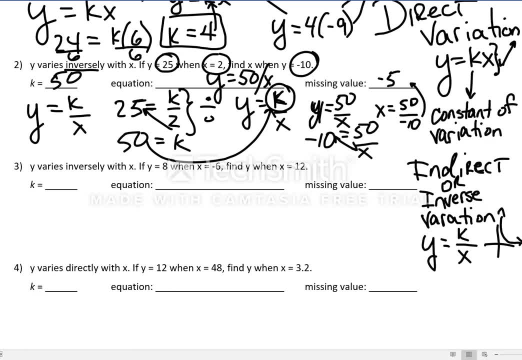 So it's really: x equals to 50 over negative 10, which is then negative 5.. So numbers 3 and 4, I want you guys to work on those. Pause the video at this moment And I'll make sure it actually gets paused as well. 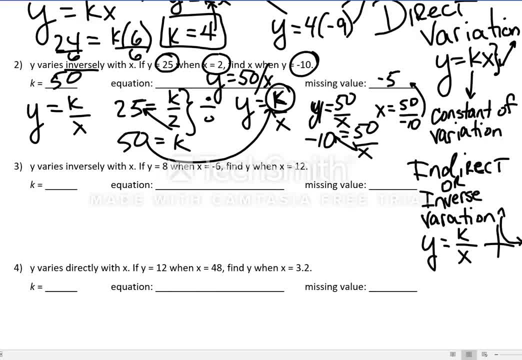 And then go ahead and write your answer down, And I will write the answer down as well. All right answers, Here we go. I'm not going to do much work because you can do all the work, But your k value for number 3 is going to be negative 48.. 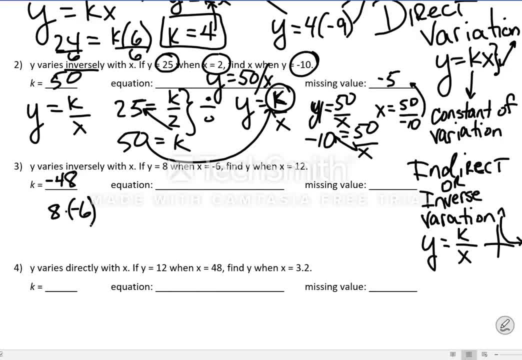 Because it's really 8 times negative 6.. Okay, Your equation is then using the inverse equation, plugging in the negative 48 and dividing it by x, And then your missing value is going to be negative 4.. Because negative 48 divided by 12 is negative 4.. 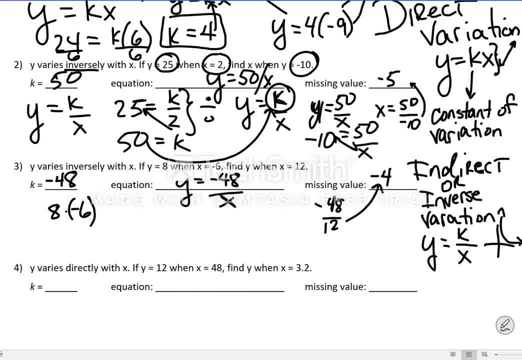 Now number 4, this is a direct equation. So therefore I'm actually dividing 12 and 48.. So it's 0.25.. 0.25. My equation. if you have 1, 4th, that is also correct.